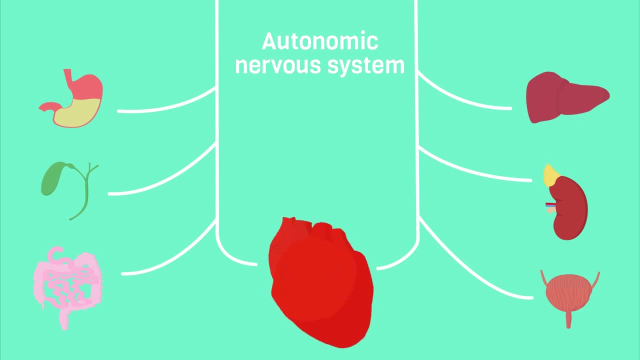 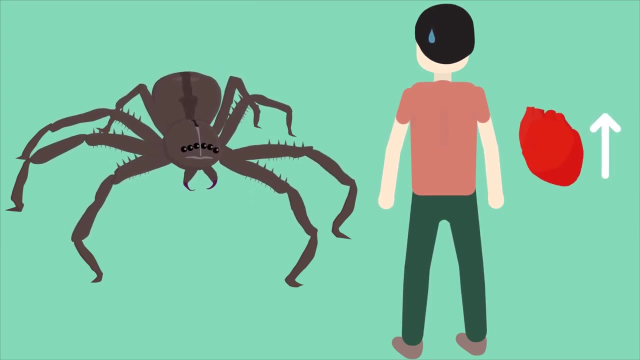 system which handles about 90% of the body's involuntary functions. The sympathetic nervous system is what kicks into gear when we are stressed or in danger. We sweat, our heart rate goes up and the interval between our heart beats goes down. We produce norepinephrine. 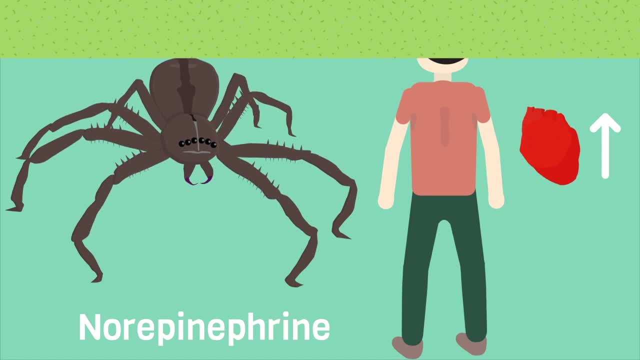 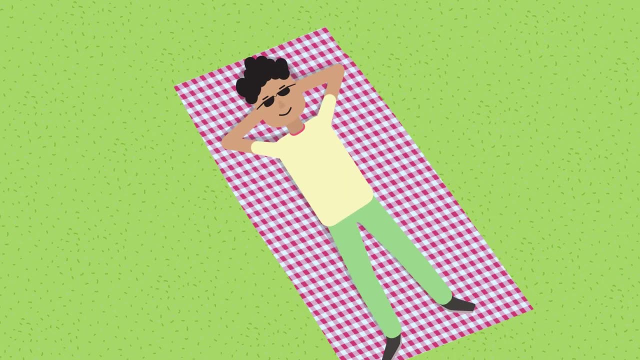 and our body is primed to either fight or flight. The parasympathetic nervous system is pretty much the opposite and it's the opposite. It functions like a brake. by disabling the sympathetic nervous system, Dubbed the rest and digest response. it activates when we are in a relaxed state and engages processes. 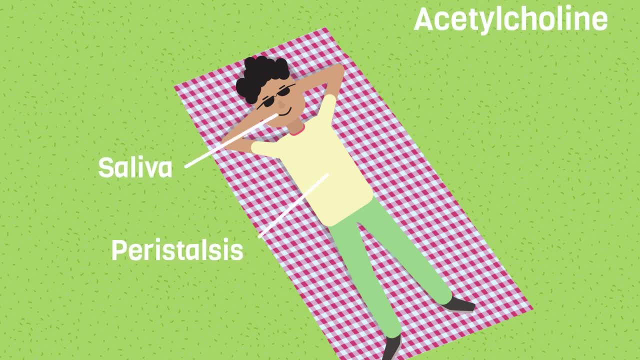 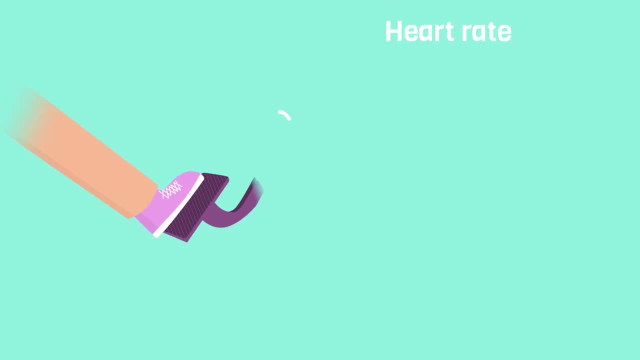 such as the production of saliva and peristalsis. It uses acetylcholine to make the heart beat slower and with greater intervals. When imbalanced, they therefore produce high HRV through a more variable heart rate. The more variable your heart rate, the more you are able to readily. 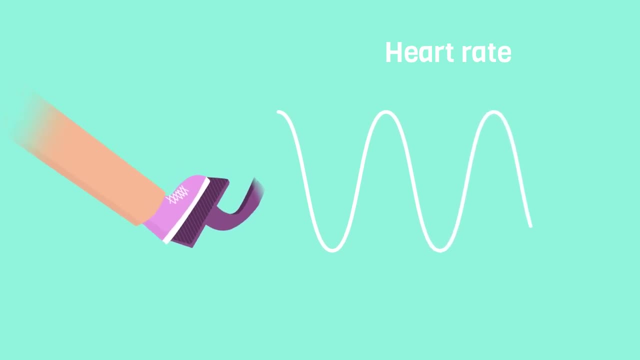 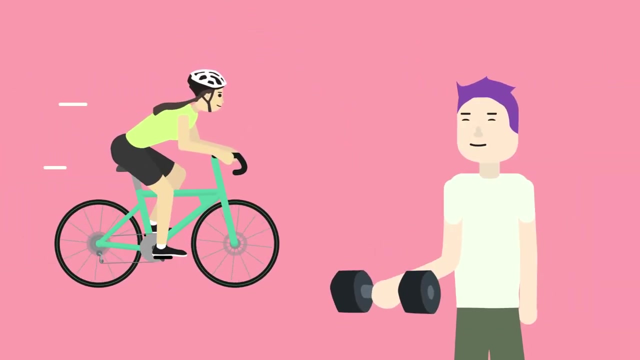 respond to your environment and switch gears between these two systems. HRV is used as a health marker. It generally decreases with age. High HRV is an indication of cardiovascular health, fitness, willpower, calm and positive emotions and your ability to handle stress and exercise. 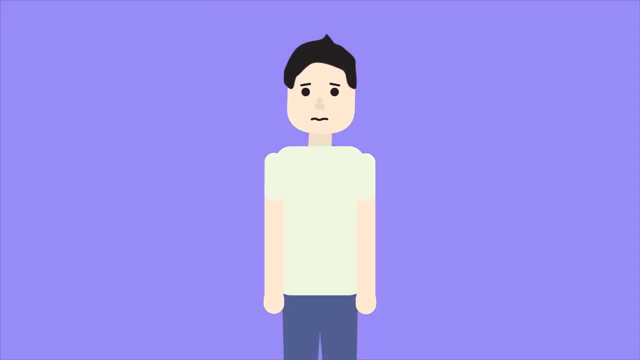 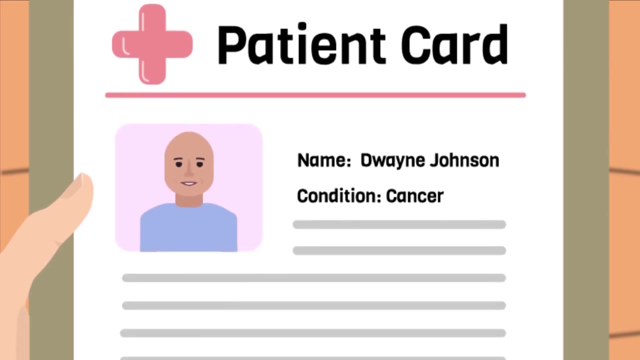 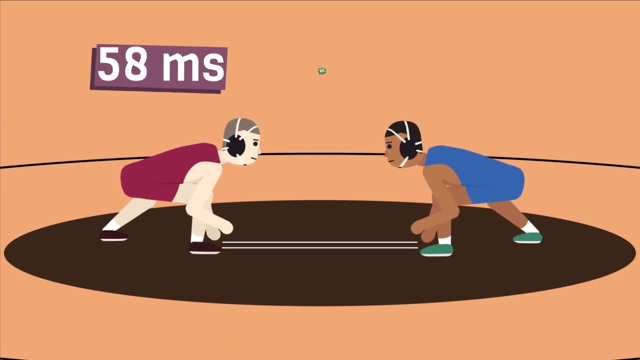 Low HRV is related to inflammation, chronic stress, chronic pain, depression, cancer and low emotional flexibility. HRV values have actually been used to predict injury recovery and cancer outcomes. One sports scientist has been able to predict very accurately the point differential in wrestling matches. 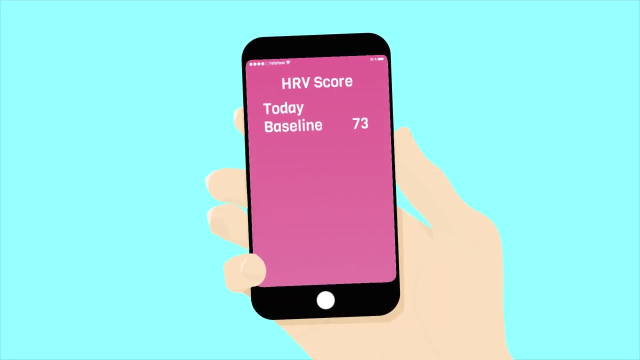 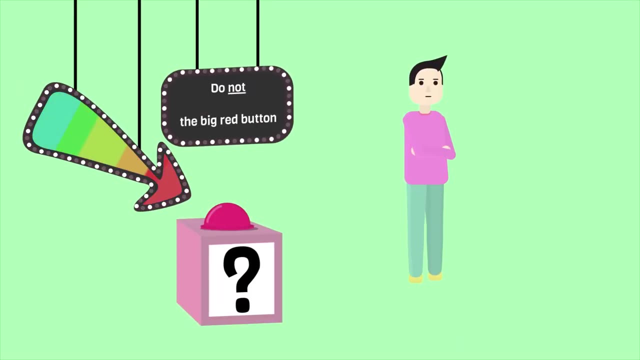 based on pre-match HRV readings. Elite athletes use daily HRV measurements to adjust their training regimen and prevent overtraining. There is also an interesting link between HRV and willpower. HRV is a huge predictor of persistence and self-control, and it increases when exerting self-regulation. This mechanism 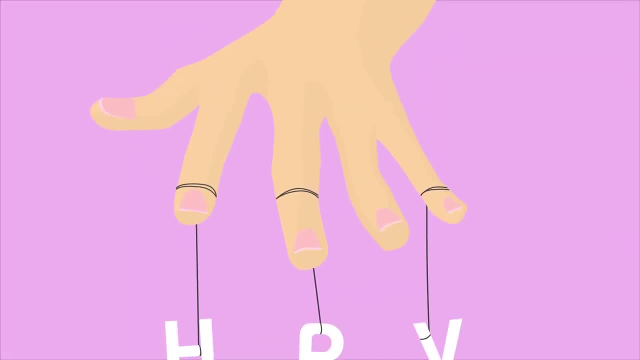 is called the pause and plan response. By changing our physiology, we can manipulate our HRV, and the way we do this is through breathing and what is called resonance frequency breathing. Combining this breathing with biofilm and radioactivity makes our breathing more responsive and developing expressed patient confidence. we can then have more potency, while 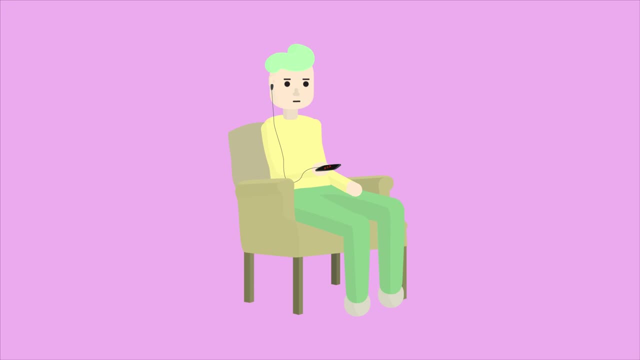 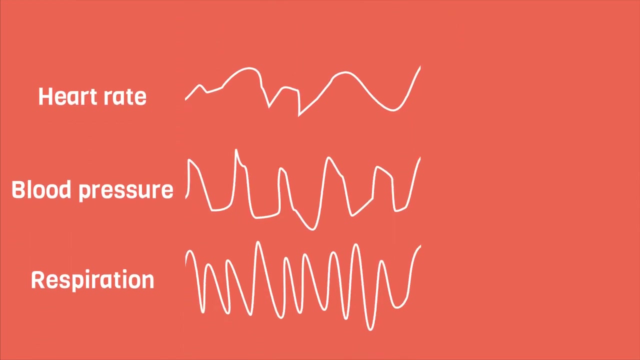 effect device to monitor your hrv in real time is called hrv training. by slowing down your breathing, you can activate the parasympathetic nervous system and raise your hrv, which causes your heart rate and blood pressure to synchronize with your respiration, resulting in a state that the 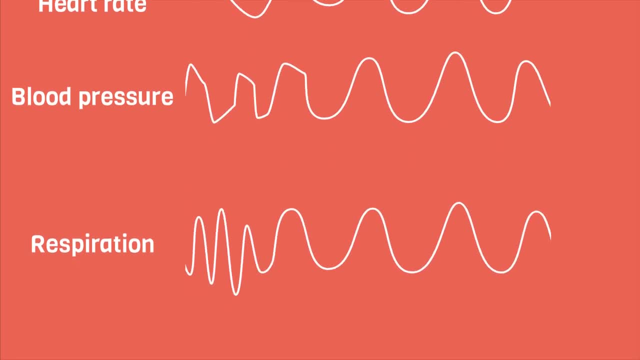 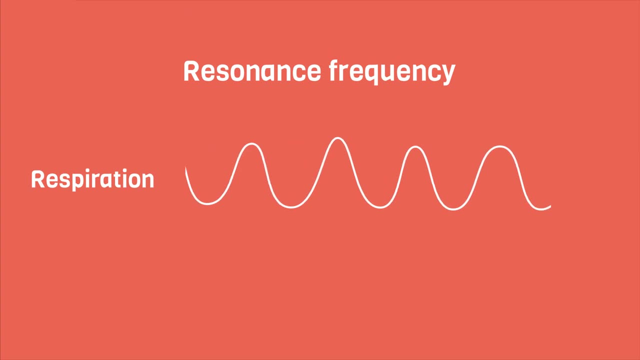 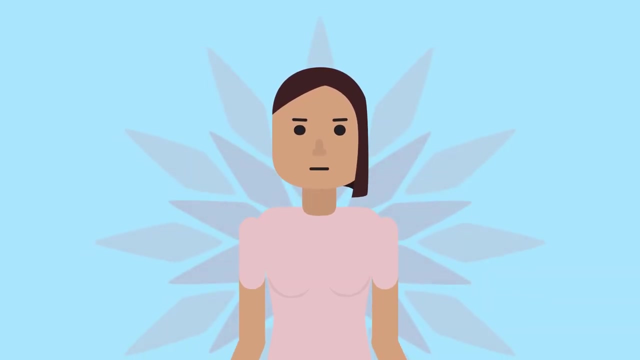 heart math institute calls coherence the optimal rate of breathing that produces coherence and increases your hrv the most differs from individual to individual and is called your resonance frequency. for most people it will be around 5.5 seconds. doing minimum 10 minutes of this breathing every day, you can develop the skill of producing a state of coherence at any given moment. 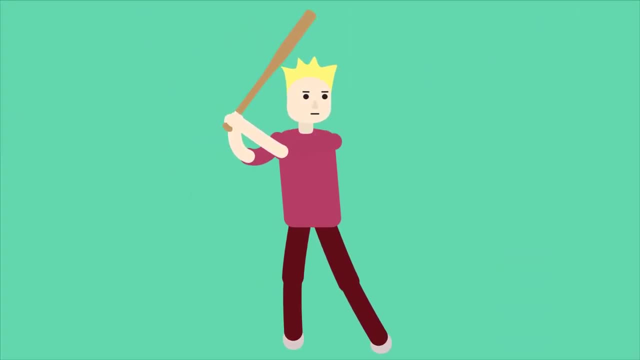 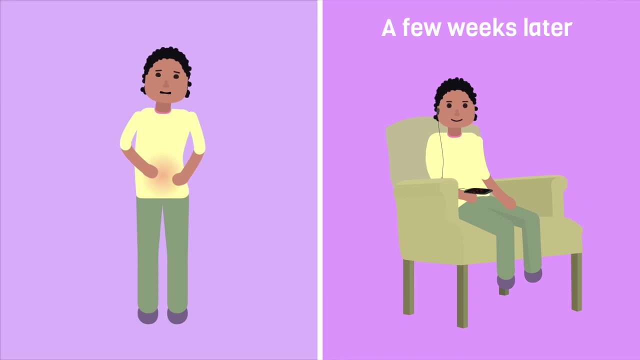 activating the state, you can get into the zone, so to speak, and increase your performance for single actions such as swinging a golf club or hitting a baseball. hrv training has shown to be incredibly beneficial for kids with overactive sympathetic nervous systems and resulting belly aches. after a few weeks of daily training, they show massive improvements in their base. level of breathing and their breathing will be much better than before with hrv training. it's a great way to plan hrv and are able to function much better. some autoimmune conditions related to the gut have been helped by this type of training, as well as our gut permeability is. 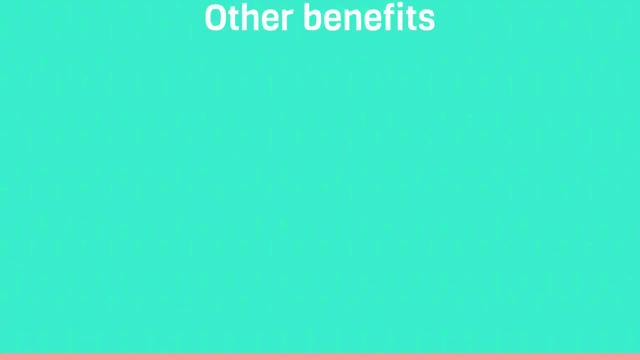 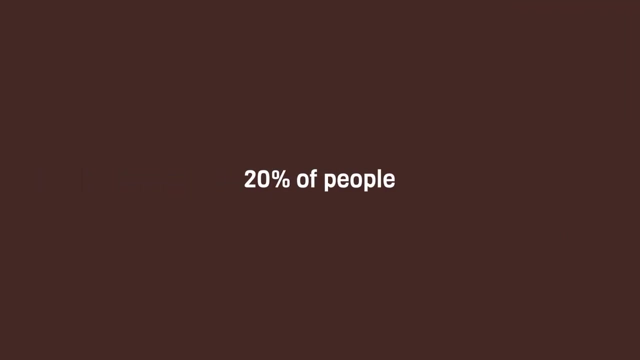 closely related to our parasympathetic nervous system. other benefits of hrv breathing include pain management in conditions such as fibromyalgia and chronic muscle pain. it can help with asthma, depression, hypertension and self-control. it's also great for stress management. around 20 percent of people will feel sleepy from following this breathing rhythm, which makes 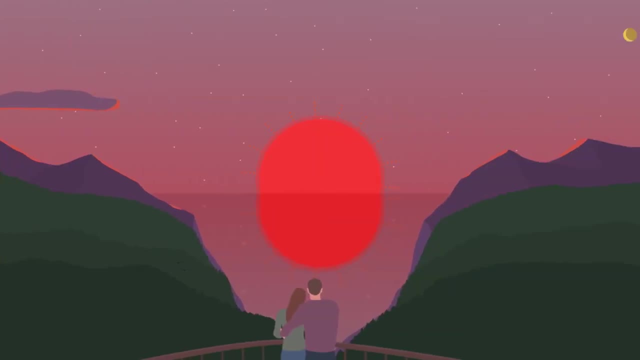 it a great tool for falling asleep quickly at night. if you want to experience this state of coherence, i've created two videos for you to practice this breathing. one is suitable for the morning or day and looks like this, and one is made for nighttime, with minimal blue light, if 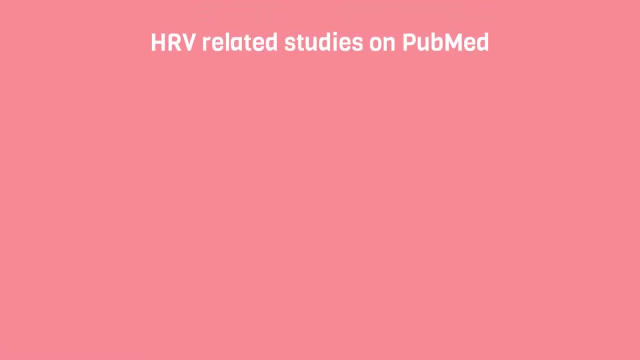 you'd prefer doing it right before bed. the interest in hrv has increased substantially the past decade and several consumer technologies have emerged to help measure your personal hrv metrics. the most accessible way to accurately measure your hrv is to get a polar heart rate chest strap and connected. 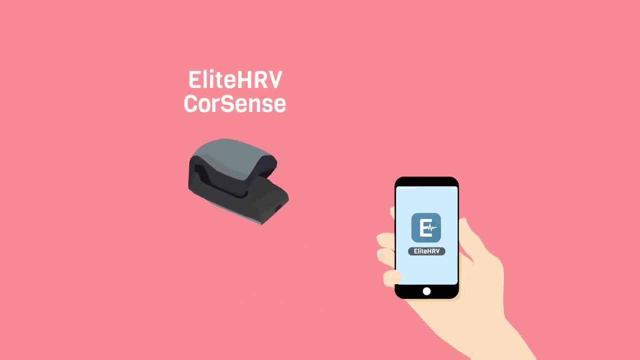 app called Elite HRV. Elite HRV also sells a device called CoreSense which you stick a finger into to measure your HRV. The previously mentioned HeartMath Institute has created the M-Wave device and the Inner Balance Sensor to provide biofeedback as you perform HRV training. The 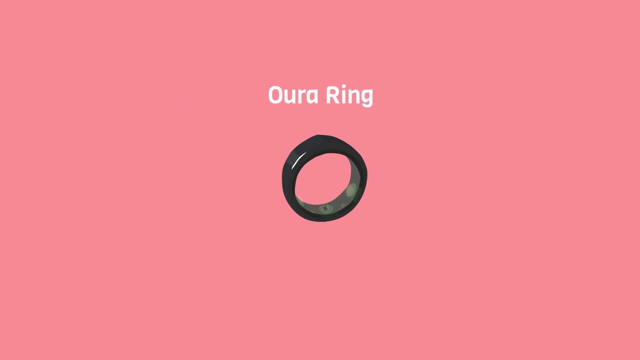 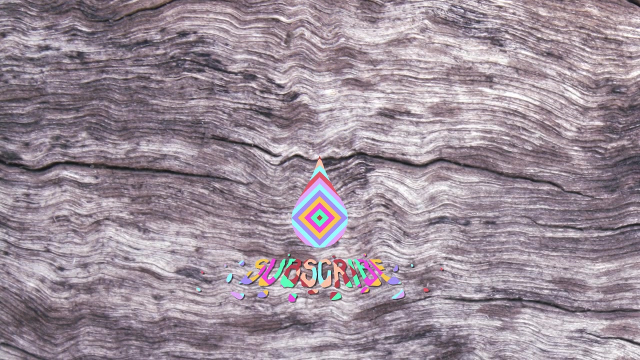 Aura Ring is a sleep tracker that shows you an average HRV value from your night of sleep. I've added links to these in the video description below and also links to a few more resources on HRV, if you're interested in learning more about the subject. Thank you for watching this video.